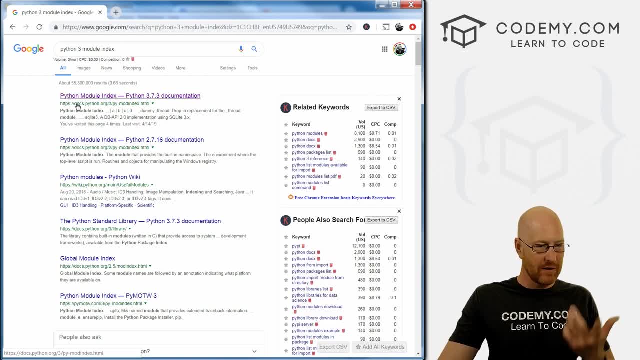 index. you get this right up at the top. it's: this is the Python documentation. It's the Python module index for Python 3.7.3.. If it's a different version number by the time you watch this video, Python is always updating and stuff, So that's no big deal whatever. 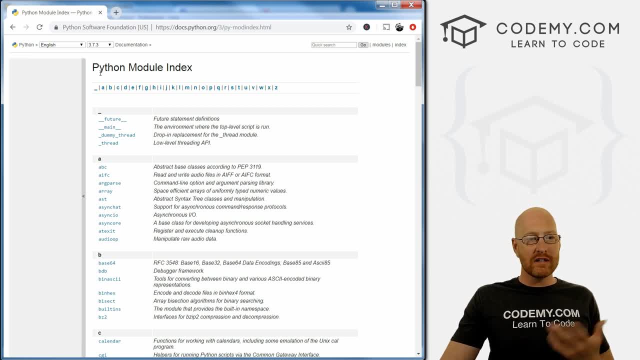 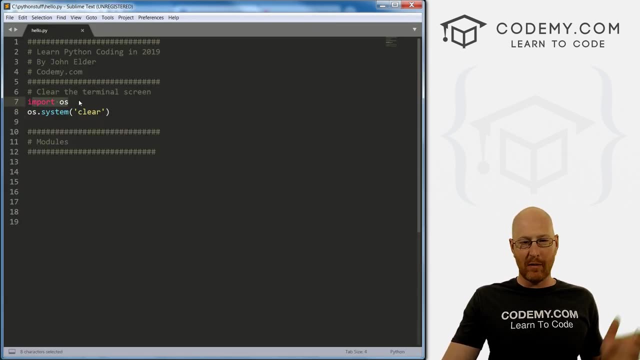 it is. just take a look at the, the latest one, And here we have this, my module index, And this just lists all the modules that come with Python And you can- I mean that means you can- use them without installing them, Like we did see earlier here. we just referenced them at the top. we imported 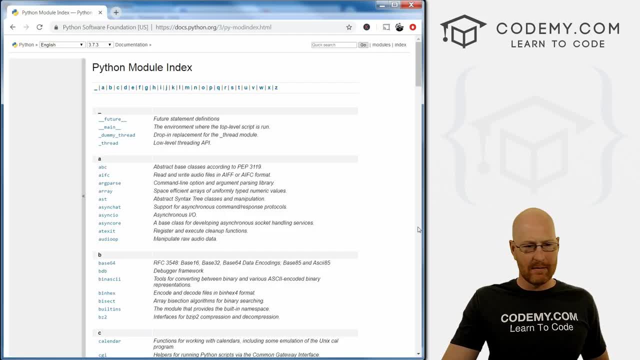 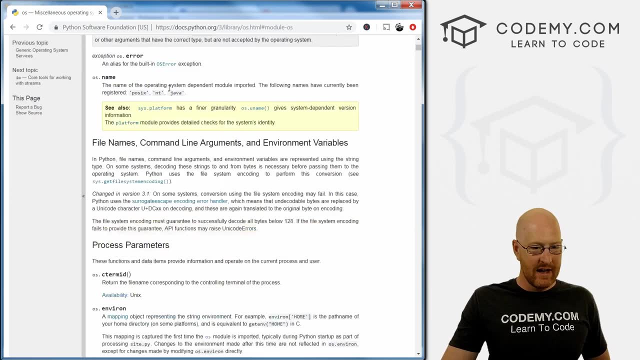 it and we can use it. So let's take a quick look at some of these. If you scroll down here, for instance, we go down to Oh, we can see: here's that OS, one that we've been using, And what have we been doing with it? we've just been 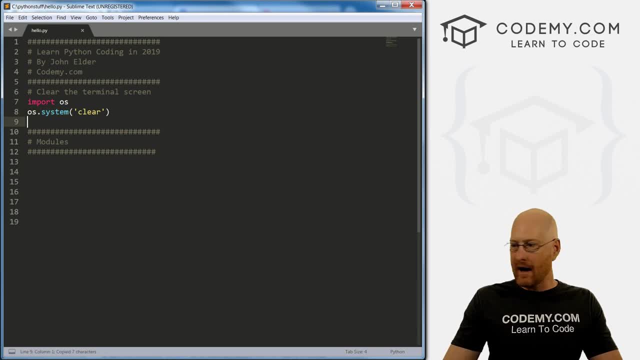 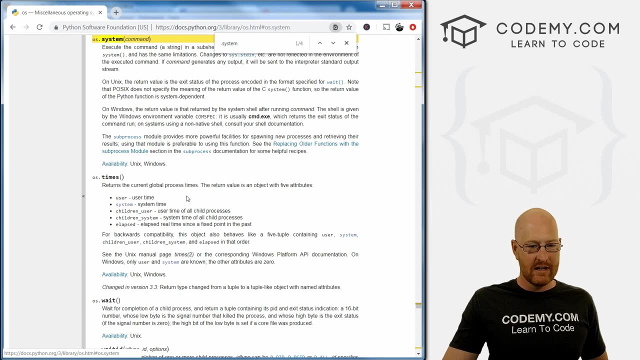 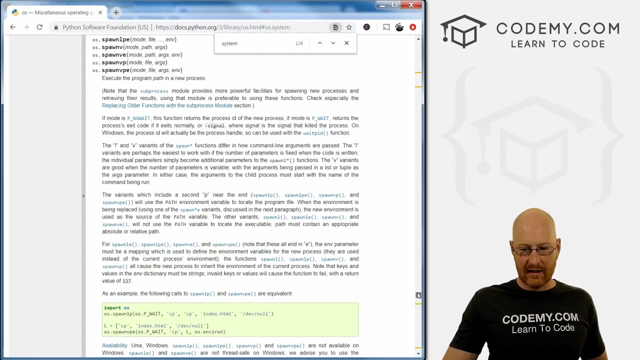 Using OS dot system. So if I want to copy this and just search for that, I can see, boom, right here is OS dot system. If we click on it we can read all about it, what it does and all the good stuff, And you can see there's a lot of stuff on this page, right, Some of 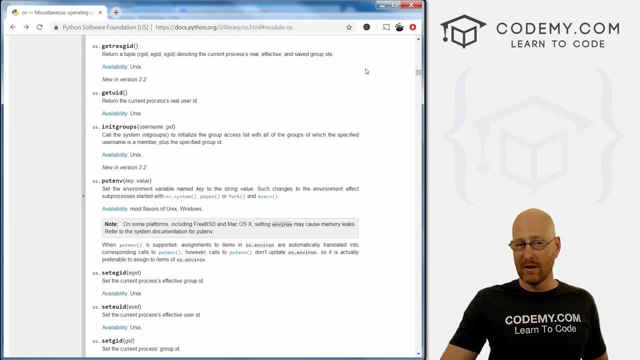 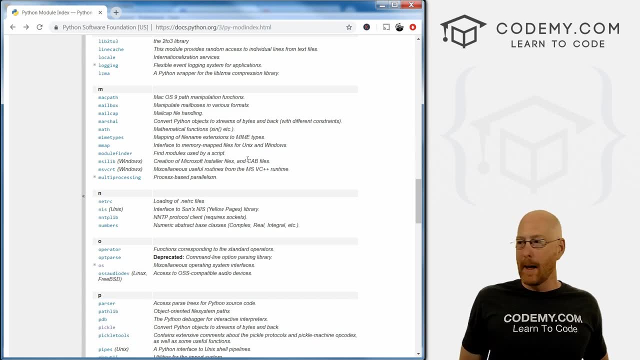 these have a lot of information, a lot of things they can do. Some of them are very short and small and there's not a whole lot there To learn, but they're all kind of cool And I really recommend that you sort of just spend. 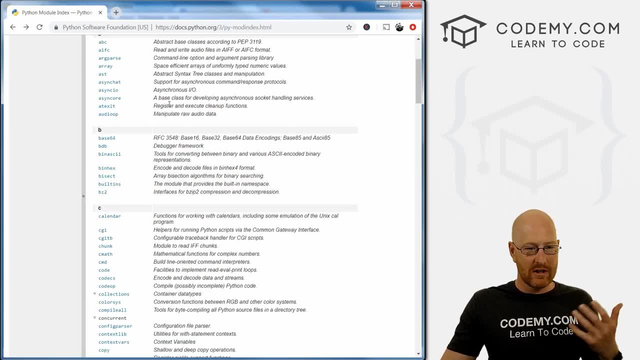 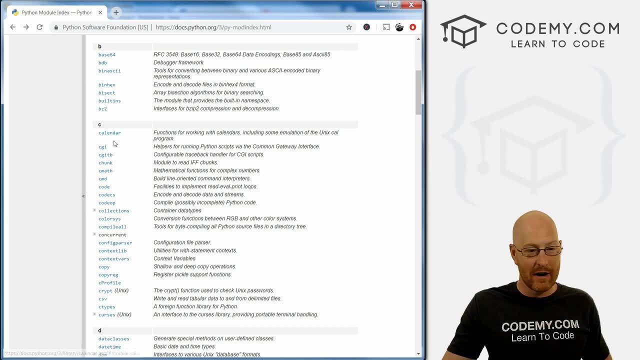 some time going through here and just looking, just seeing first off, just kind of browse through and see if anything grabs your eye. It's something you're interested in. If you need to use a calendar, well, there's a calendar module. maybe you want to read about it. Let's. 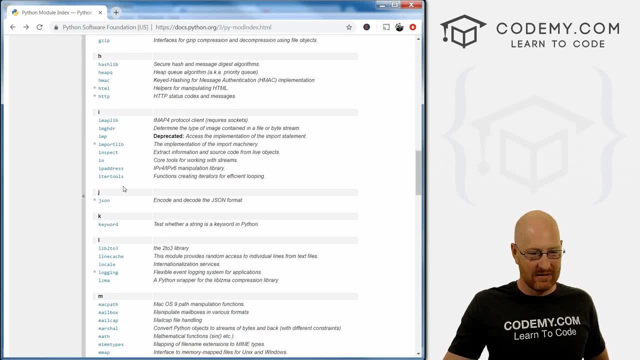 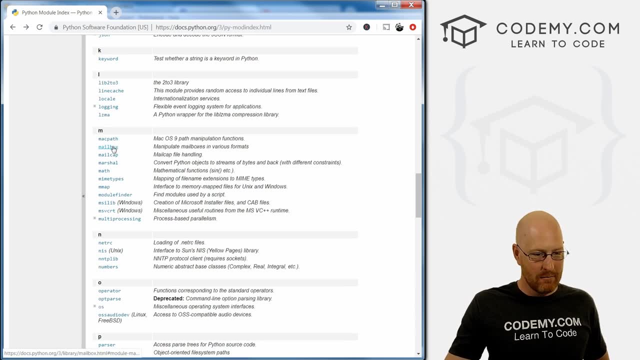 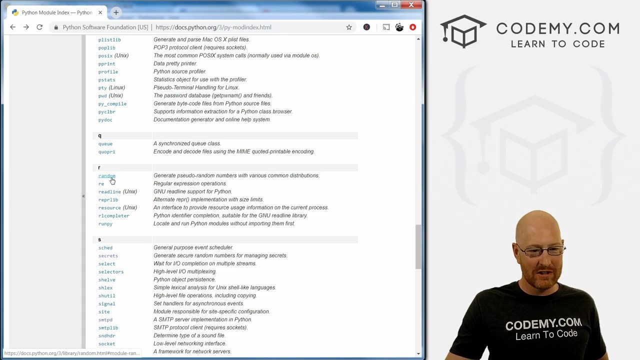 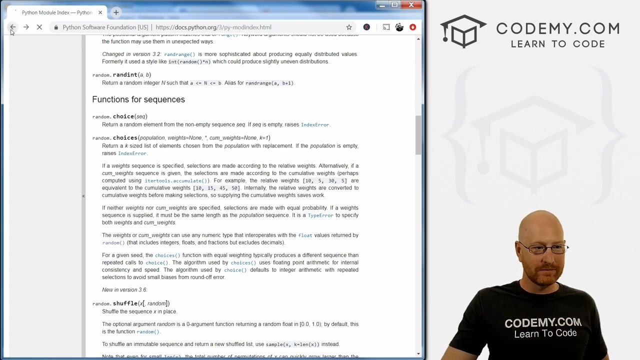 see, we just kind of eyeballing this. There's a JSON. if you're going to be using JSON, JavaScript object notation: mailbox Pickle. I have no idea what that is. If you want to use random numbers, there's the random module. There's all kinds of stuff that helps you create random numbers Very. 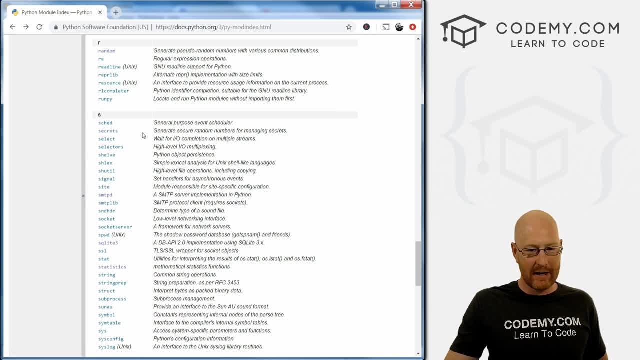 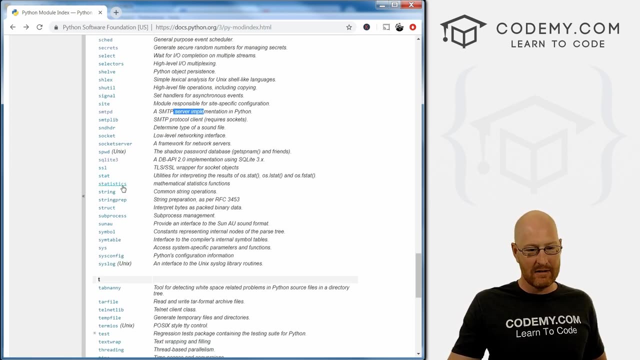 cool Secrets for generating more secure random numbers for SSH keys and things like that. I think SMTP, This is a email server. I want to learn how to use that statistics stat. you're into math stuff? Very cool. Check out the statistics And you. 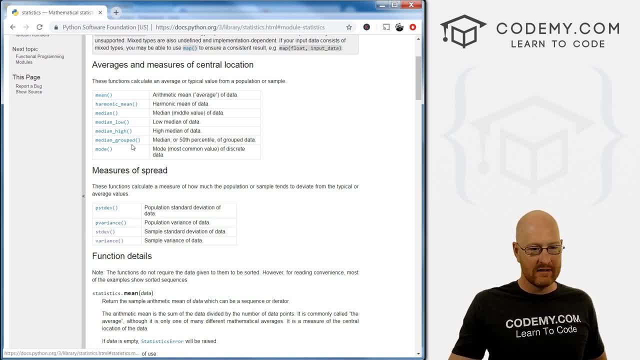 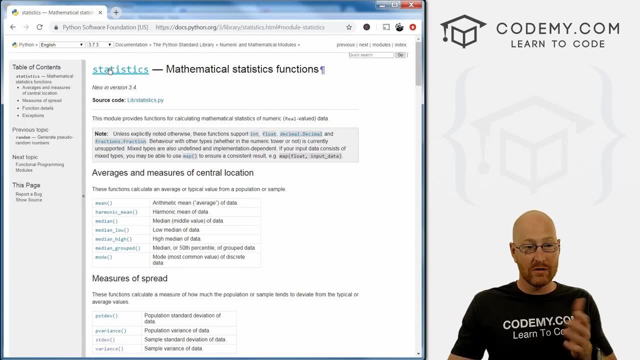 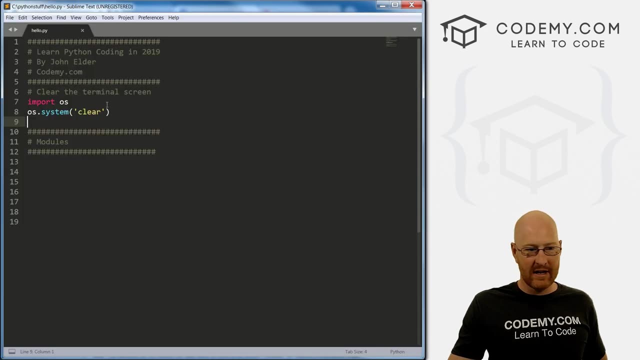 can see the statistics has mean median. I can get standard deviation and variance very easily. Very, very cool, And we already know how to use all of these things. You know to use, for instance, statistics. you just would come over to your thing here and you 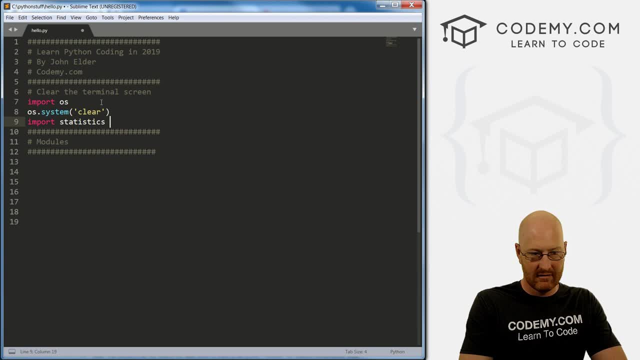 would go import statistics Right and that's it. Now you can start using it as per the instructions on that screen. So very powerful stuff and very easy to use. So spend some time going through there, read through some of them And I recommend you really find something that you're interested. 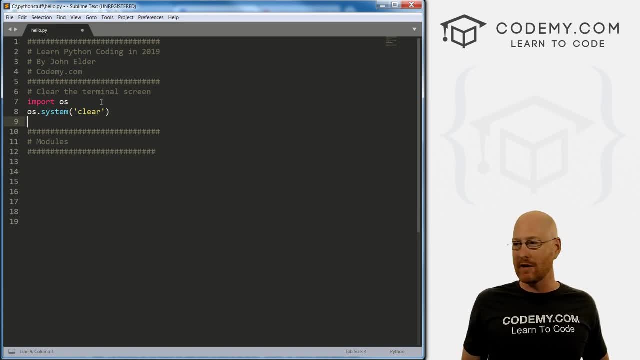 in there and learn all about it, everything there is. if you're interested in random numbers, learn everything you can on that page about random numbers and then start playing with it And that's you know how we learn these things And very, very cool. So those are. 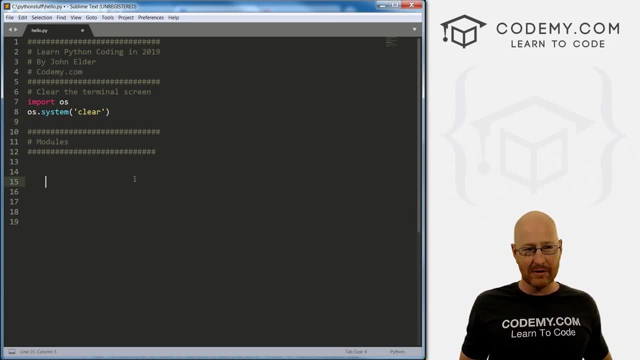 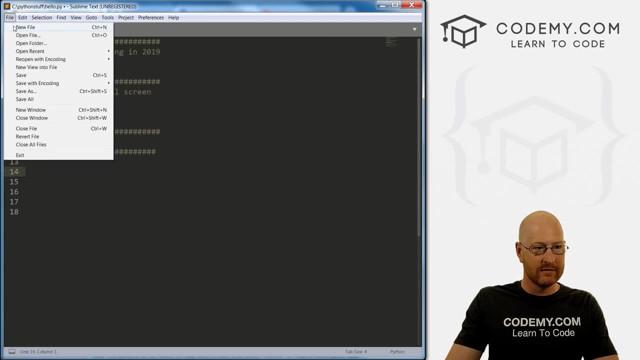 the built in modules And, like I said, we can create our own modules And it's actually really, really easy. So I'm gonna just come up here and create a new file And let's create that namer. We do a. 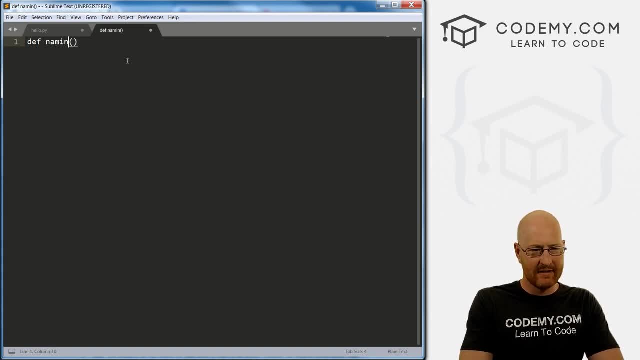 namer- What do we call it? name it. I will do a namer, create a namer module And right off the bat I'm going to save this as. and we want to save this in the same directory where our other file is. So we're in this Python stuff directory And I'm going to go. 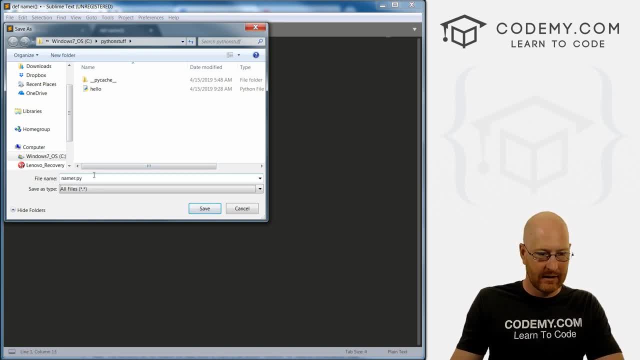 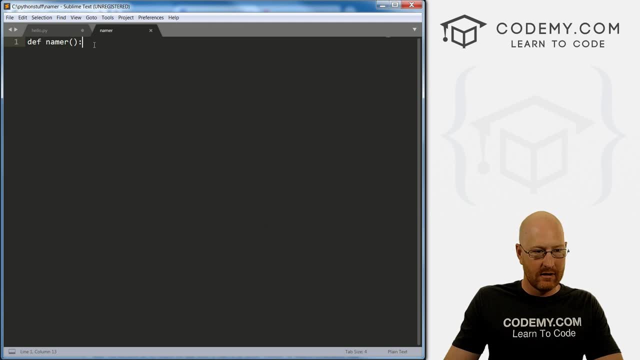 ahead and I'm just going to call this namer pi. Make sure this is Python. Okay, it looks like it did not get saved as Python. Let's try it again. File save as: delete this one Namer dot pi. just type it in. All right, there we go, The colors changed And now I 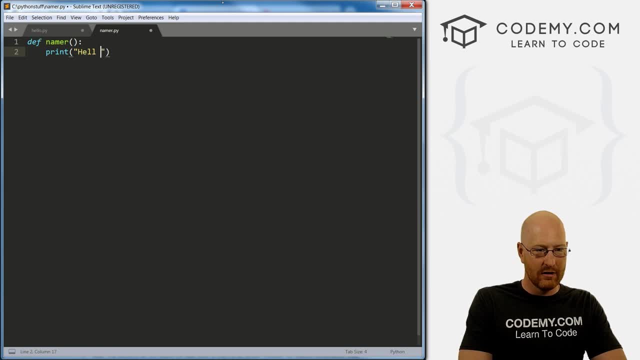 know we did return before, but I'm just going to go ahead and create a new one And I'm going to print out Hello, Their name, and of course, we need to pass in name, Alright, so I'm just going to save this, And this is just a Python script we've just created, right? 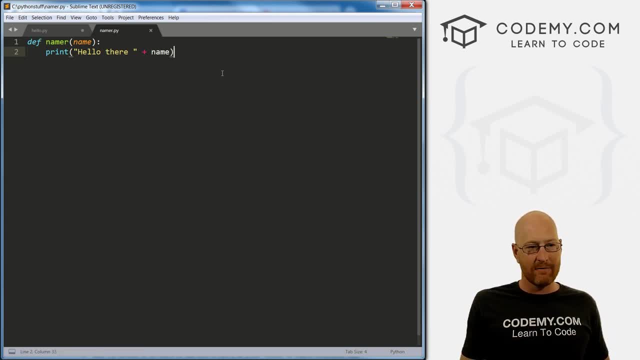 just a regular Python file And it has this function, the namer function. And you know what? I'm going to change this to name it. Yeah, Name it, Nam it. I don't know. save this Now to use this. we can import this just like we've imported everything all. 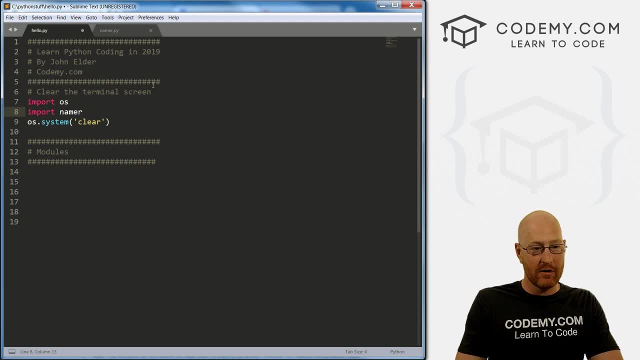 our other modules import And we call namer the name of the file. right Now we can call from namer dot, name it And then we can pass in john Alright. so from namer, which is the name of the file, namer dot pi. we want to reference the name it function, which is: 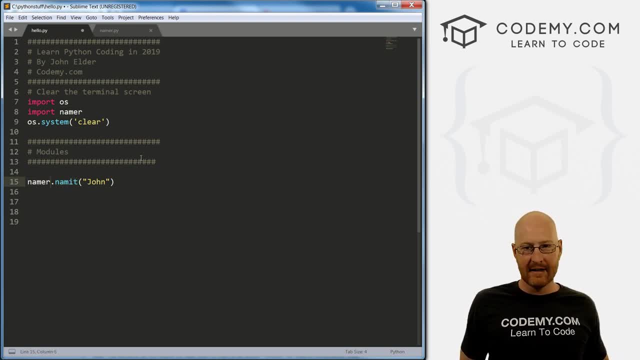 this right here And you notice we've just put a period, a dot. this is a very object oriented type of thing to do that you can do with Python. When you want to use something inside of something else, you just dot and then put the name of the thing. So if we save, 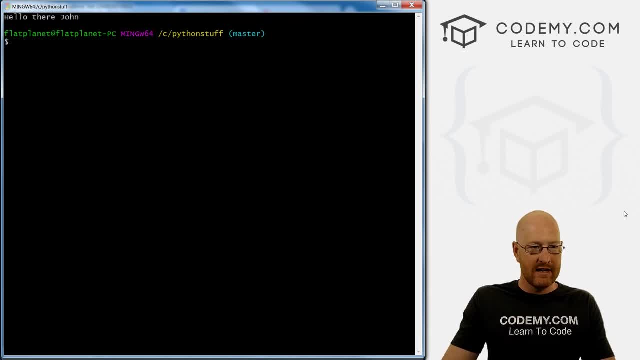 this: come back over to our command line and run this. This is Hello there, john, And we could, you know, change this to Bob. save it, run it again. Hello there, Bob. Now, that's one way to do it, And that's definitely a way to do it. 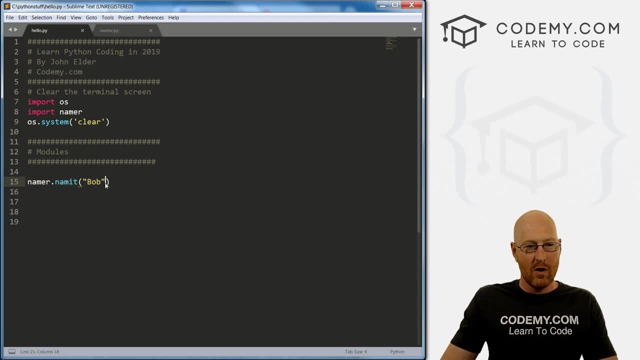 But this can get a little confusing. from namer name it. we can actually change this around up here. we can go from namer, import, name it And then get rid of this. we don't need that. So from this line we're doing the same thing: we're importing, But here we're. 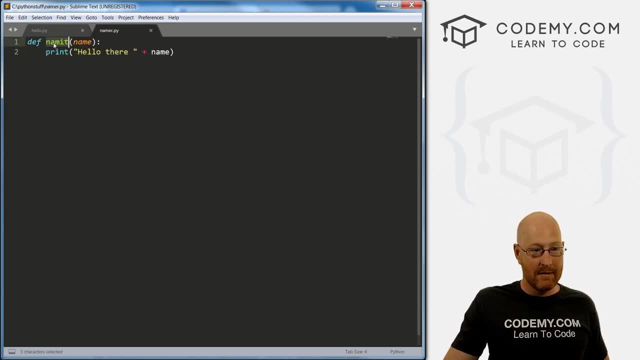 importing something specific, In our case this name it function. we're importing name it from namer And now, from now on, we can just reference it by referencing the function name, like we would always right. So if we save this, actually let's change this to: 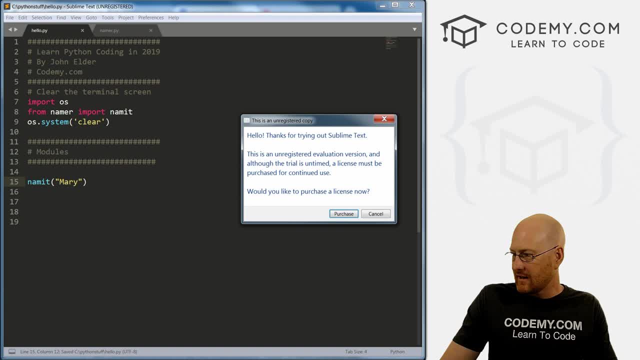 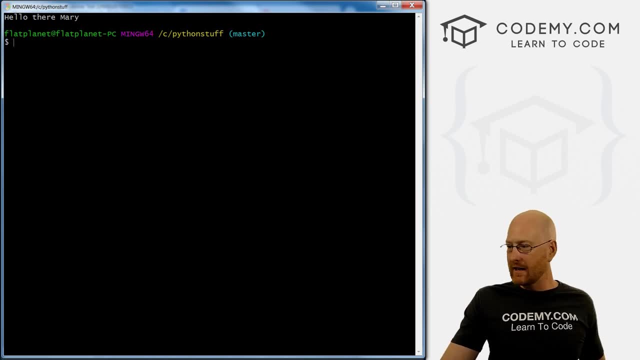 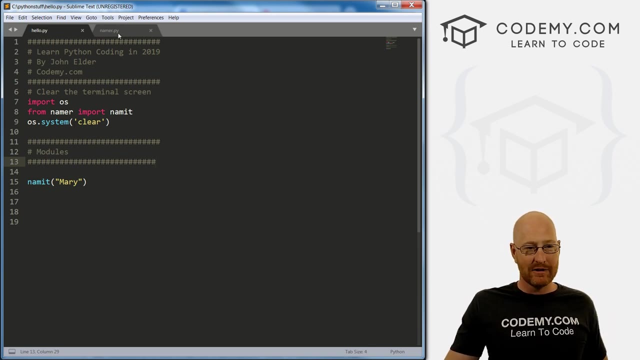 Mary, Save it, Run it. Hello there, Mary. Very cool and very easy. Now there's lots of different ways you can bring in code from other programs. treating them as a module and just importing them like that is probably the easiest in my mind And very cool So. 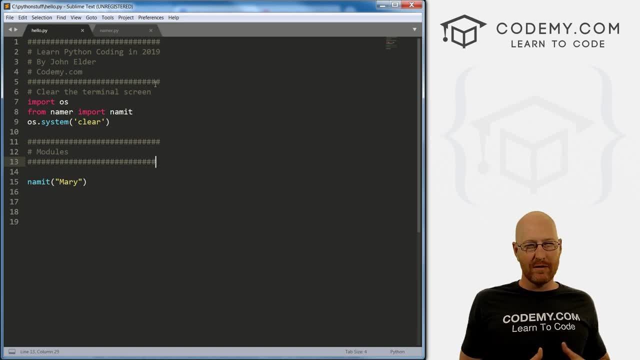 you know, it's a good idea to break apart your code. So if you've got a big function- that's you know a lot of code- you might break that off into another file and then just import it like you would any module, And it helps keep your code cleaner. You know, and it's. 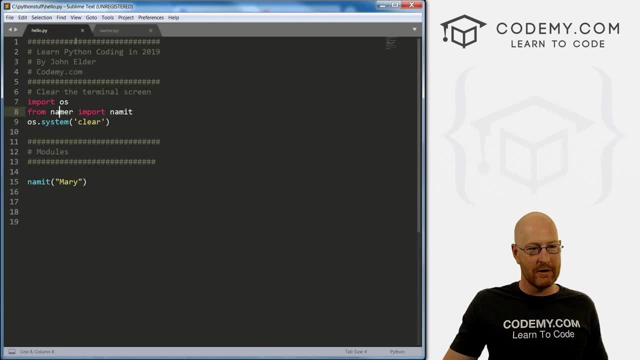 it's obvious what we're doing here. we're from namer, which is in this directory, just importing this name. it function. Here there's a placeholder variable. we're passing Mary into that placeholder variable and then running the function. 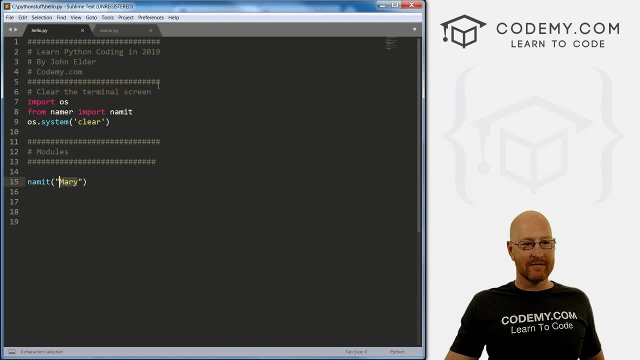 And it returns this print escape. So pretty simple but very, very powerful And it's just sort of a way to extend things. And you know, like I said, break up your code or you can use Python's built in functions or modules. I should say from that page we looked at. 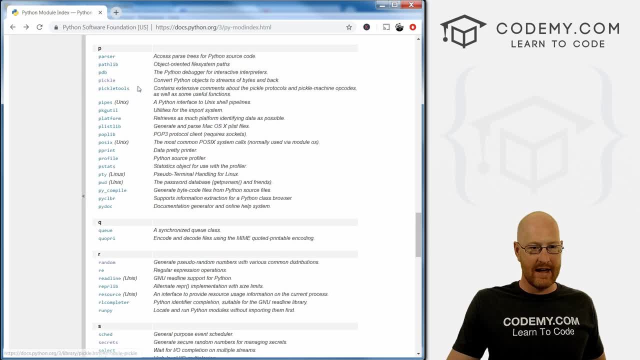 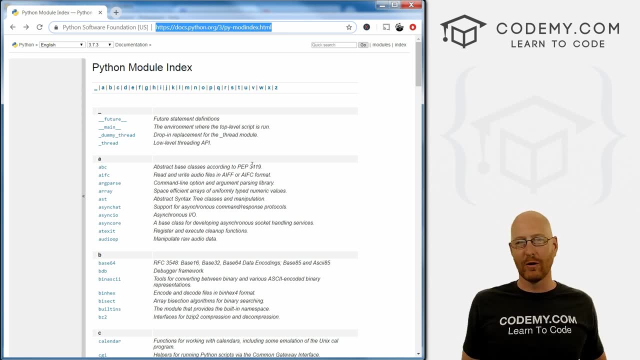 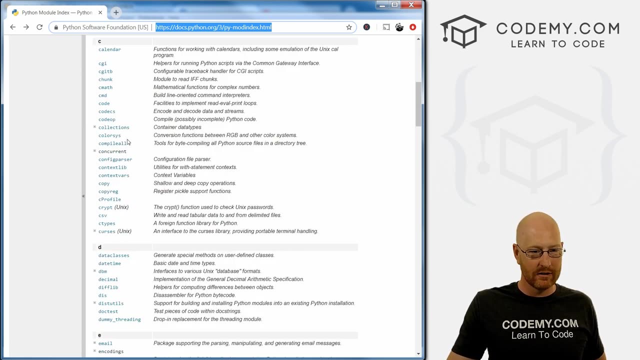 and be sure to take a look at that. It's at this URL right here. I'll put a link to this in the video below. or just go to Google and type in Python three module index and you'll get this thing. But check it out. There's a lot of stuff in here And some of it's boring. 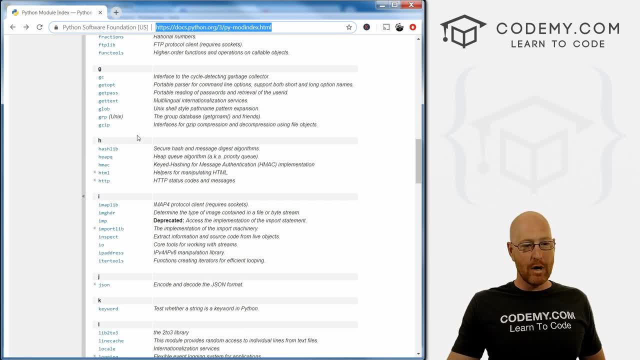 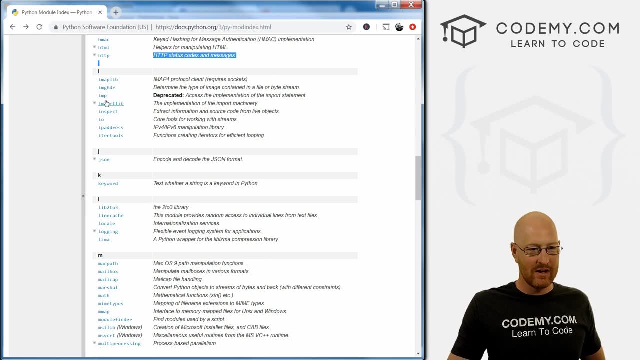 some of it's stupid. Most of it you'll never need, But help us from manipulating HTML, HTML status codes. Very cool, very interesting stuff, All kinds of cool stuff And, like I said, read through these and something might catch your eye, something you're interested. 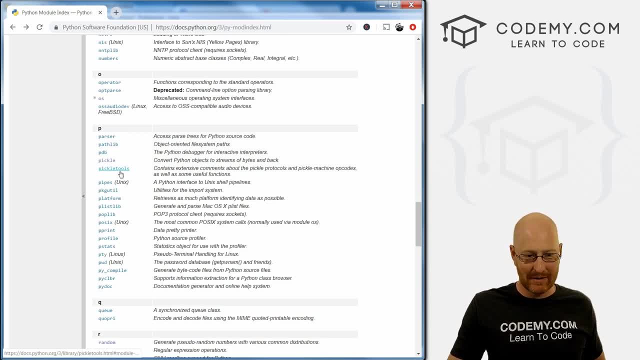 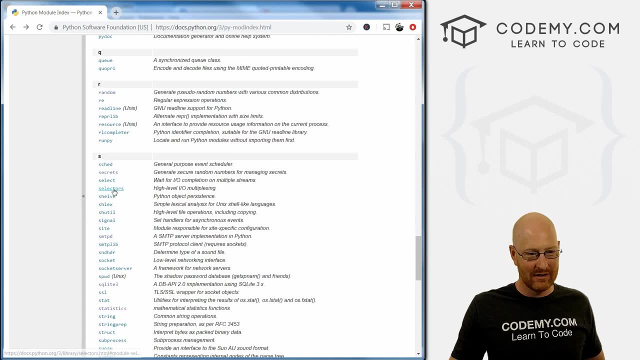 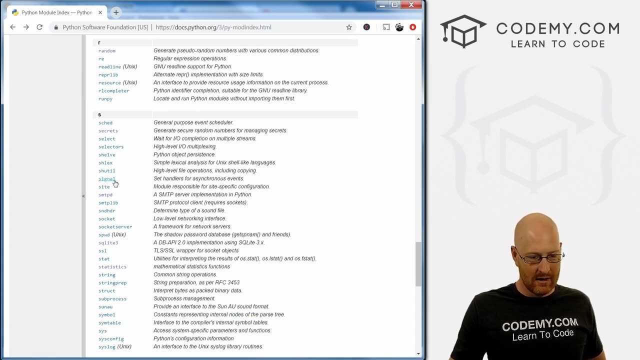 in right. Look up pickle tool, see what the what in the world is. Let's see. Let's see Q random, that's a good one. Run pi, locate and run Python modules without importing the first. that's kind of interesting. Schlecks, socket, socket, server. SQLite three is a database. 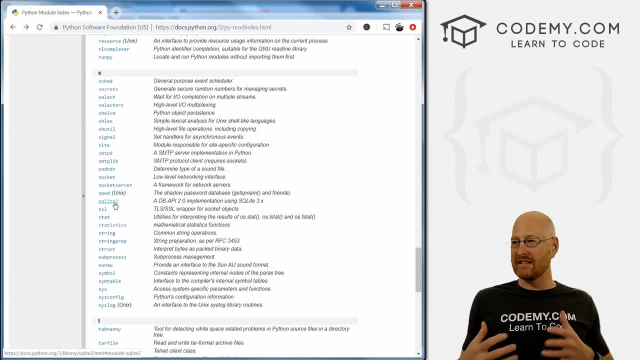 we'll probably look at that later on. That's it. It's a basic database that comes built in with Python. Oh, it's amazing. It's not good for, like, big projects, but small to medium projects where you need just a lightweight database. Fantastic. 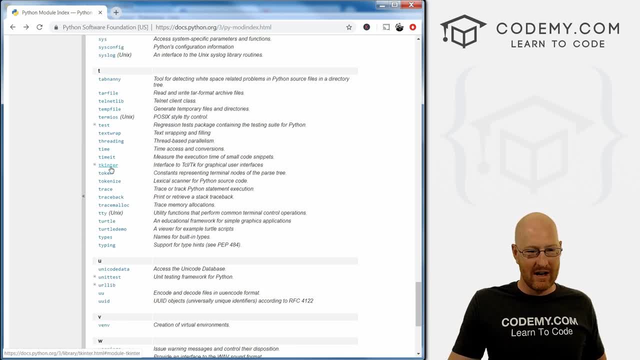 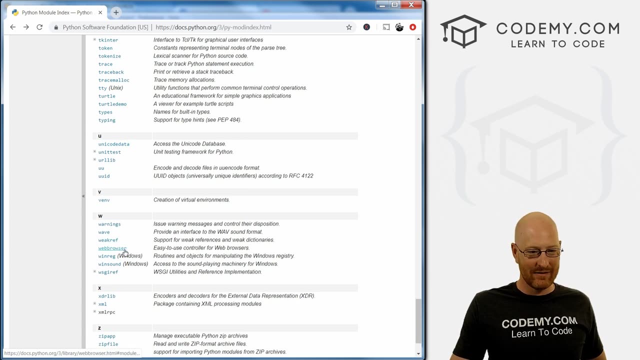 built right in right into Python, really easy to use a T kinter for creating graphical user interfaces. I've got a whole other course on that. Look at my YouTube channel. you can check that out. Very cool turtle demo. wave web browser: easy to use controller for web. 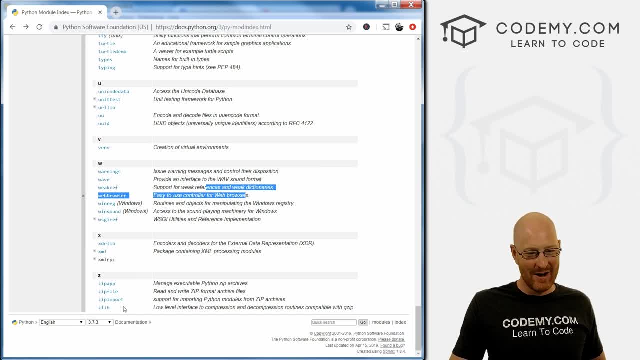 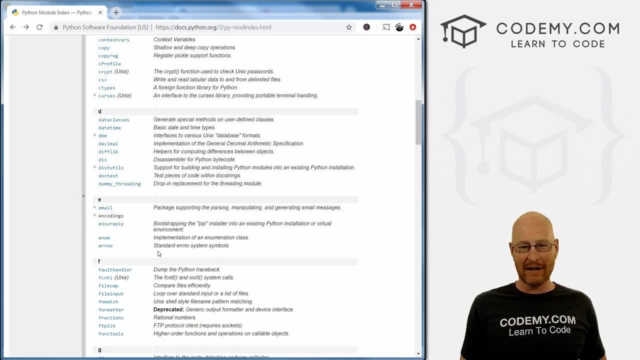 browsers. That's probably pretty interesting. All kinds of cool stuff. So those are modules. So that's all for this video. If you liked it, be sure to subscribe to our YouTube channel. Smash the like button below, subscribe to the channel and check out kodamicom, where. 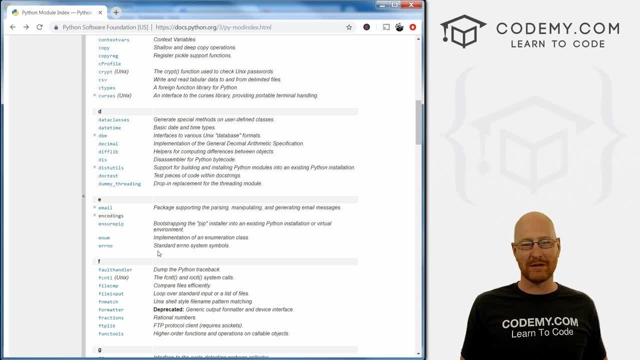 you can use coupon code YouTube to get $22 off membership. you see, pay just $27 to access all my courses, hundreds of videos and the PDFs of all my best selling coding books. Join over 50,000 students learning to code. My name is John elder from kodamicom, and we'll see you in the next video. 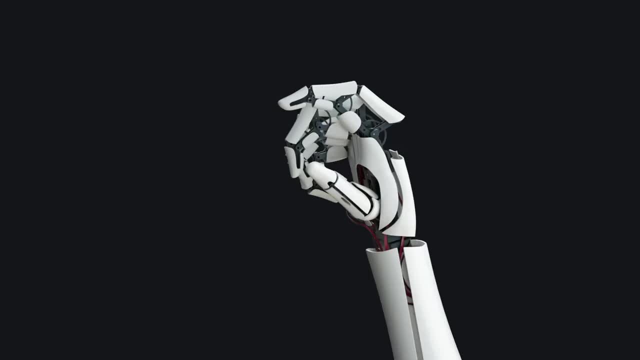 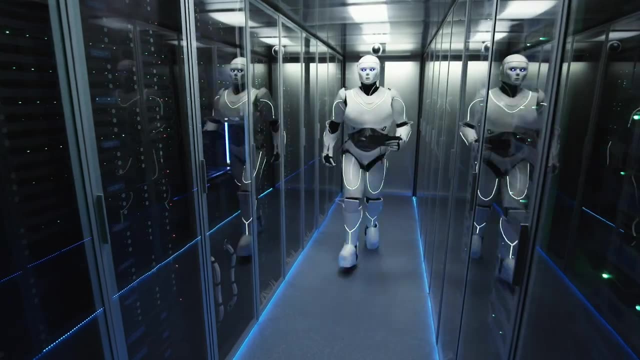 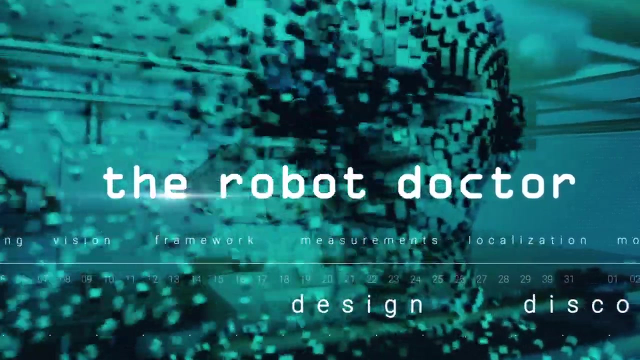 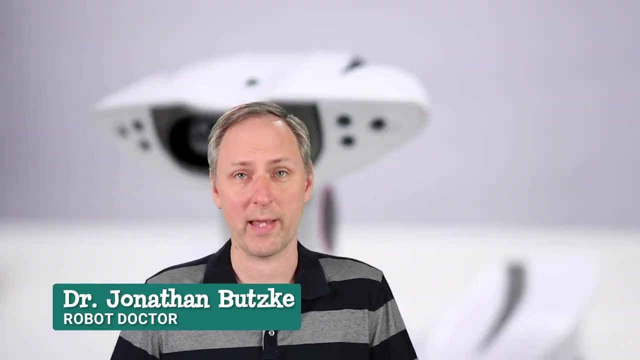 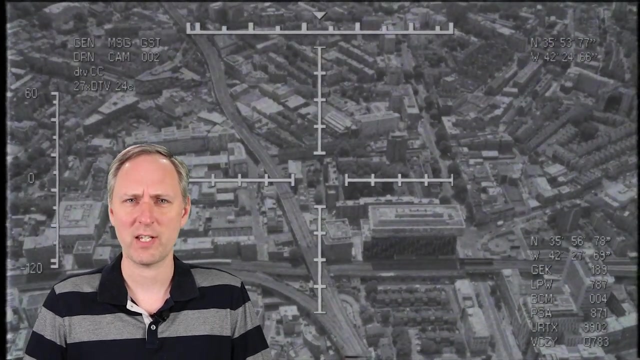 Hello, my name is Dr Jonathan Butzke. I'm not a medical doctor. Instead, I'm the robot doctor. Robots need to be able to sense their surroundings, and a common way of them doing that is with eyes made out of cameras. Cameras are handy sensors for a robot, because it allows them to see the same. 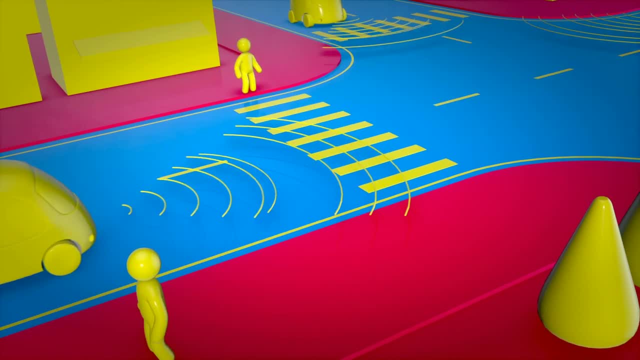 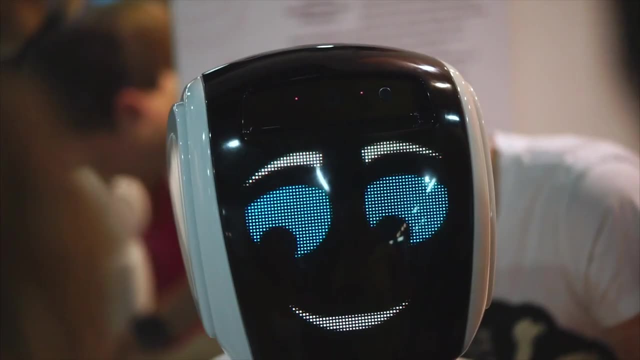 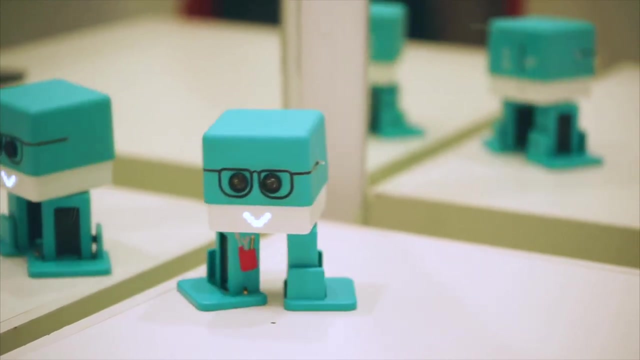 sorts of things that people see. For example, a self-driving car can use cameras to see stop signs and lane lines, A robot receptionist can see and identify people and a small mobile robot can see obstacles and avoid them. In this lesson, we'll talk about vision, How robots see things and how